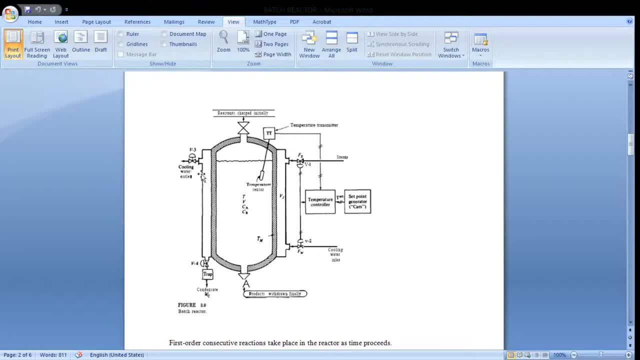 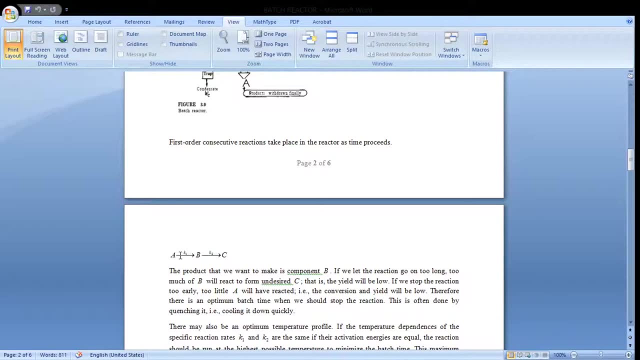 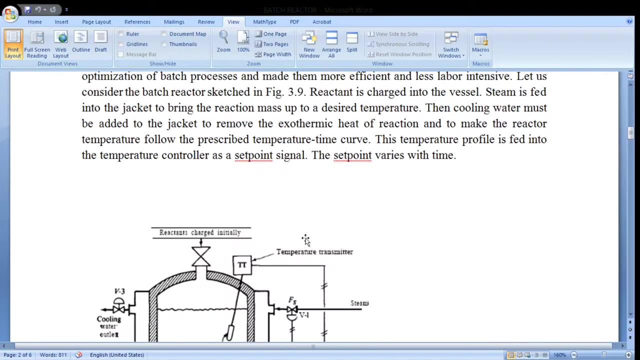 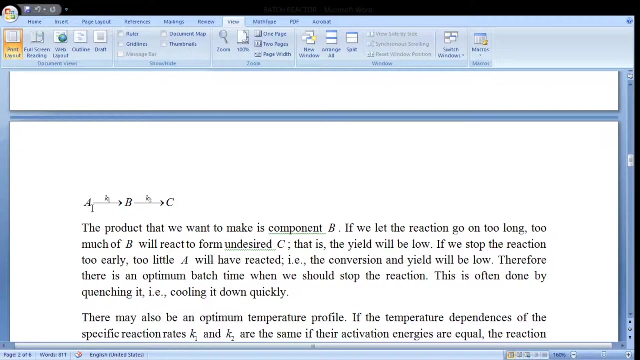 So steam is being condensed and removed, So this jacket is just to maintain the temperature. So let's say this simple reaction is taking place inside the reactor. So we say that inside this particular reactor The reaction is being this. reaction A is going to be converted to B. 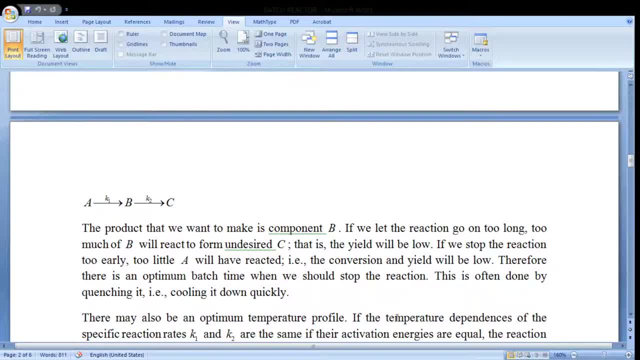 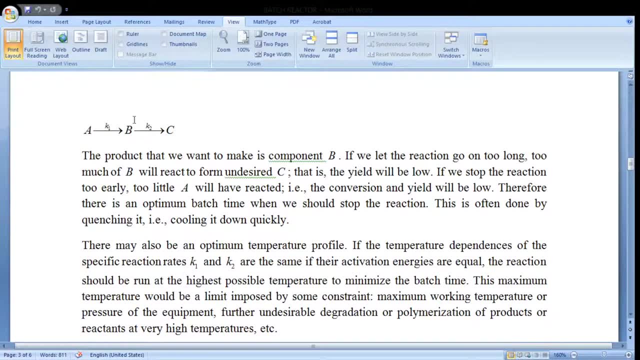 And B is getting converted to C. Now here, if B is intermediate product, Because if the desired product is C, So if you see here the product, we want to have, the B actually the product, But C is undesired product. So somehow we have to maximize the B. 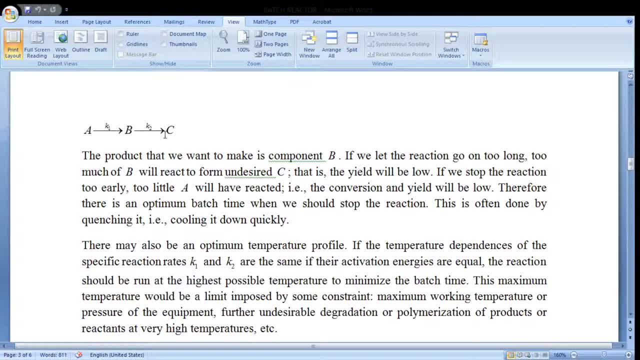 And minimize the C, And that can we see how this K1 and K2 are dependent on temperature actually. So let's say K1 is highly dependent means on temperatures, That is, have very high dependency of temperature. So we should have sufficiently high temperature. 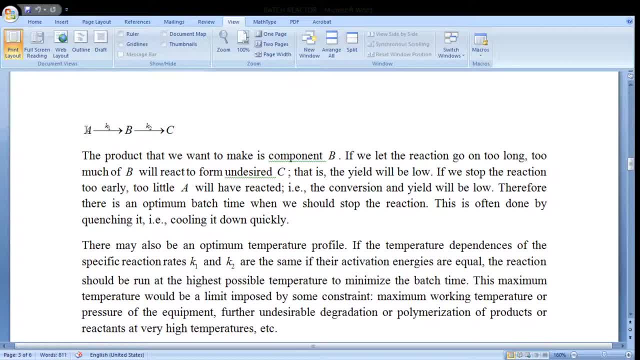 So that B can be converted. A can be totally converted into B And then reaction must be stopped In order to avoid C. Suppose B, this K1 is very slow. functions of temperature. Still this reaction need to be converted. very high temperature. 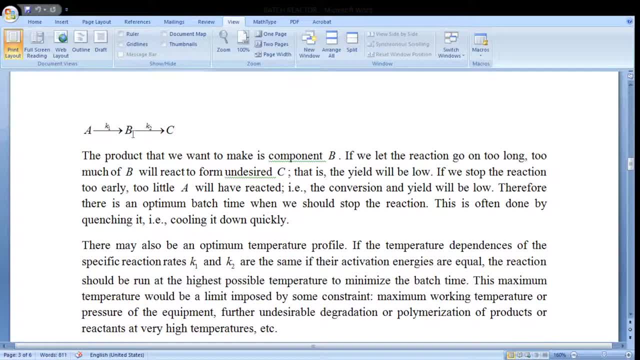 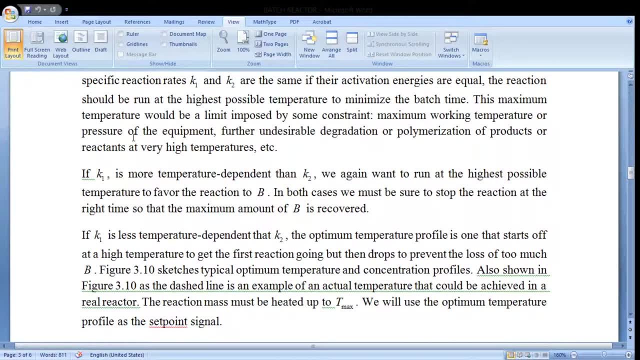 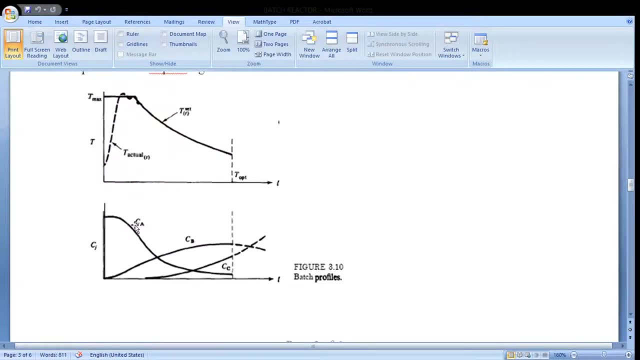 In order to have maximum of B. So depending on K and K2, the dependency, So we will get To maintain the temperature And this is how these profiles will look like that. This is the feed. The feed concentration is continuously will fall down. 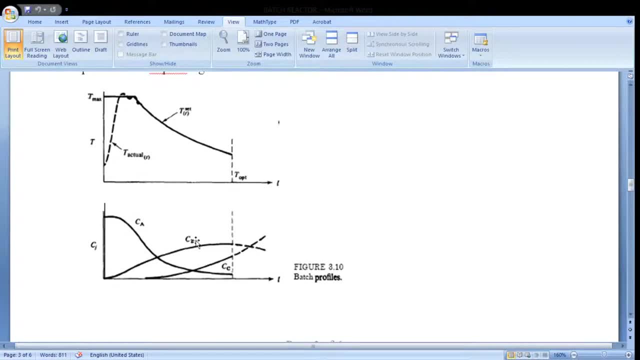 No matter how the C and B are getting produced, Now C is our desired product. So this is keeping, keep on going on and producing, And here is getting is maximum. But at the same time, if you will see, At this particular point, C is also increasing. 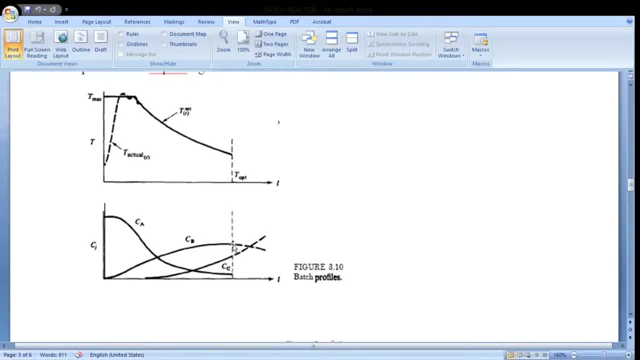 So this is not a good feasible point to have And somewhere we can end up in first batch. Can we end up here Where C is just started, C, B is just formed And after that this must be removed actually, So as soon as B is formed. 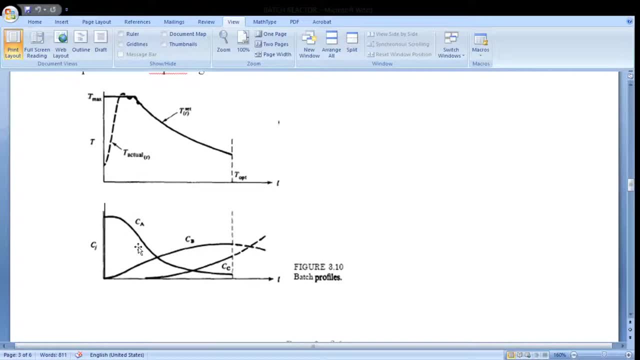 Then the reactor must be stopped In order to avoid the C actually. But for that we have to process in multiple reactors. First reactor would end up here, Then this feed would be charged to the another reactor And need the separation of B. 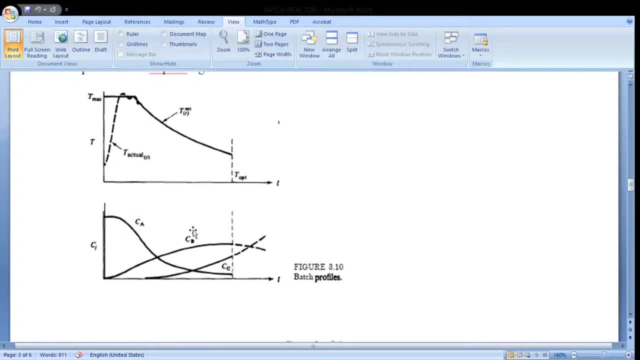 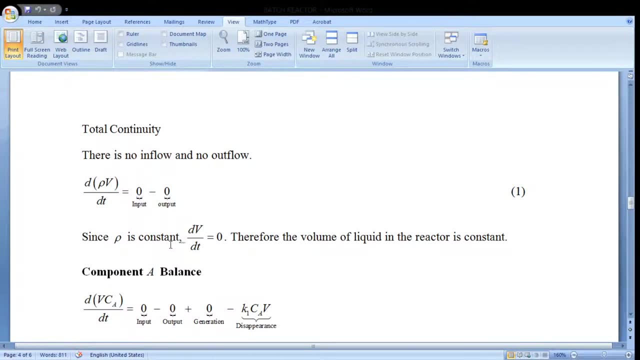 Practically is not possible. So if you write continuity equations For batch flow, Then nothing is coming in, Nothing is going out, The total mass is conserved. So D M upon D T would be equal to 0.. So this is first. 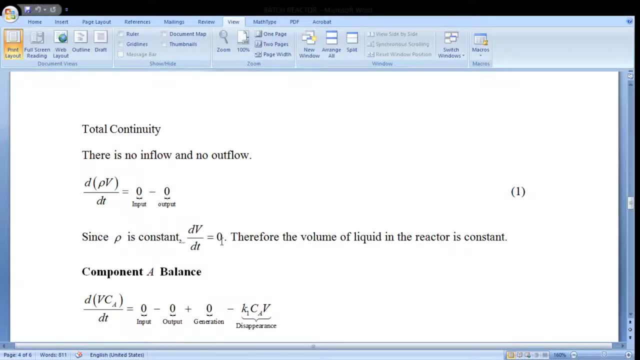 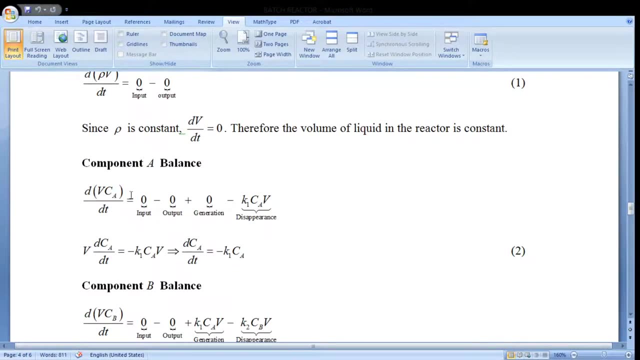 So here constant density. So D B upon D T is 0. So volume of liquid in reactor is constant. Now we are doing the component balance. So in case of V, So volume, into concentration We will give the mass of A. 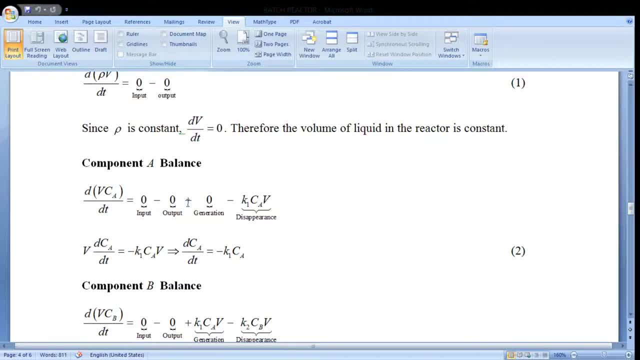 Nothing is coming in. So A is not coming in, A is not going out, A is not being generated. Only thing A is getting disappearance Means conjured By the reactions. So minus K, C, A, B. So this equation will come in this: 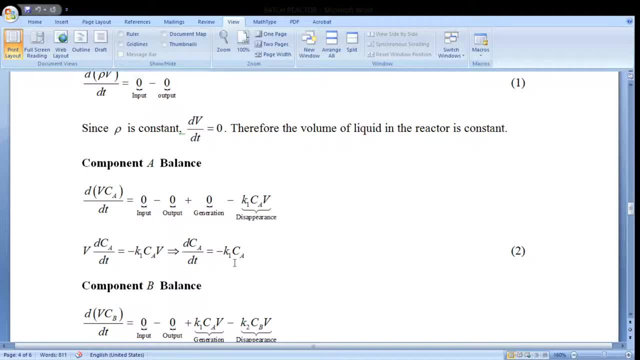 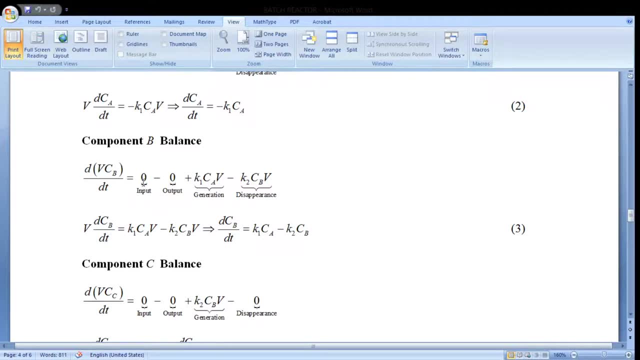 So from here we will get D C A upon D. T is minus K 1 C A. Same thing we can write component balance of B. So B is not being input, Not output. It is being generated by first reaction K 1 C A into B. 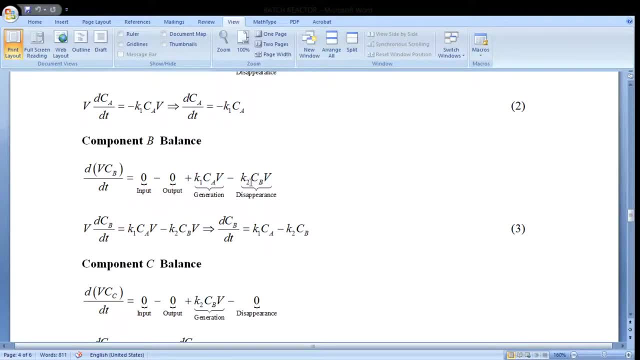 But it is being conjured by second reactions. That is the byproduct K 2 C, B, B, And for that we can write, for constant volume, case D C B upon D T equal to K 1 C A, K 2 C B. 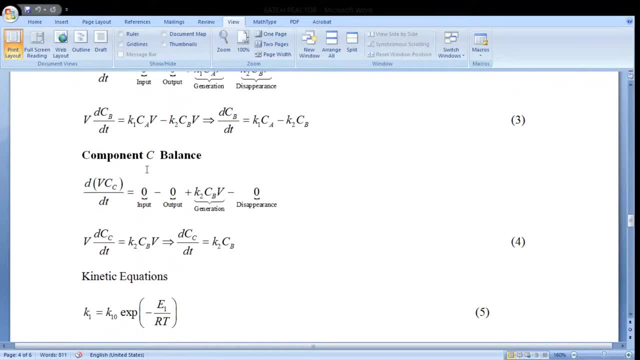 Now component C So C case. We can write a total balance equation for that For component C. So input is 0.. Output is 0.. Generation is K 2 C B, Disappearance is 0.. So you will get another equation. 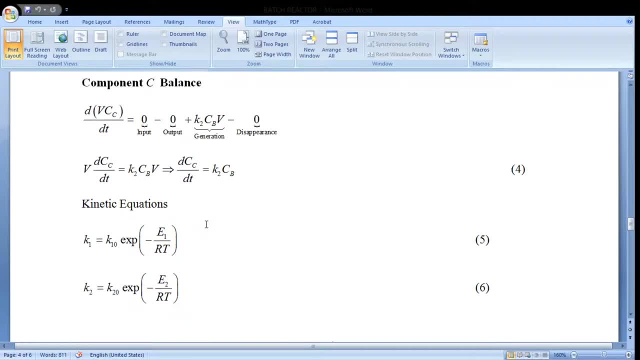 D, C, C upon D T equal to K 2, C, B. Now kinetic equation, So Arrhenius equation: We will get K 1 equal to K 1, 0.. Exponential minus E 1 upon R T, K 2.. 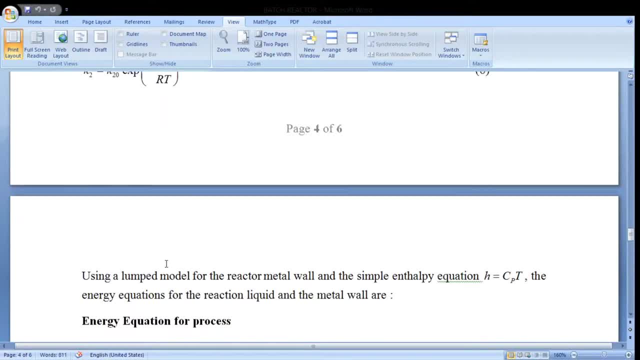 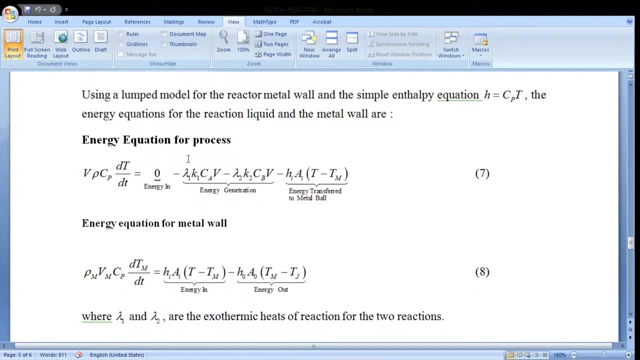 K 2, 0.. Exponential minus E 2 upon R T. So these are kinetic equations for that. After that we can write the energy balance equation for that. So this is total energy of the system. Nothing is coming in, No energy is being supplied. 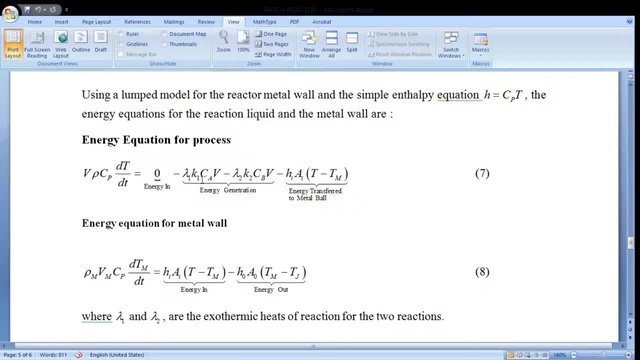 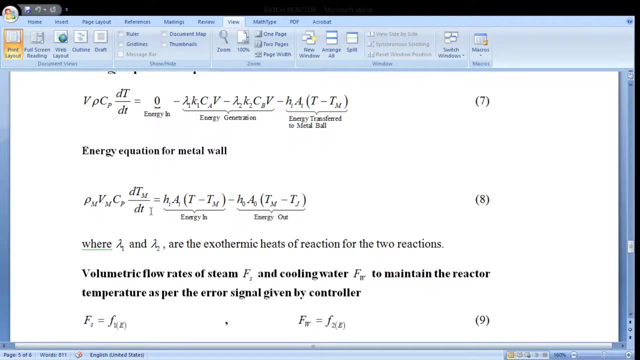 This is the energy that is generated by both the reactions here, And this is energy transferred to the metal ball, actually From the reactor to the metal ball. Now, energy equation for only four metal balls. So this is energy accumulation between the metal ball. 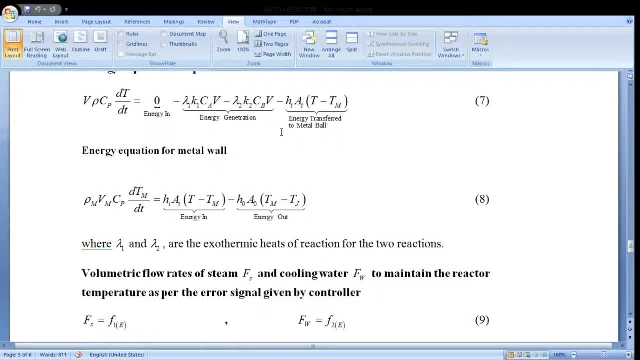 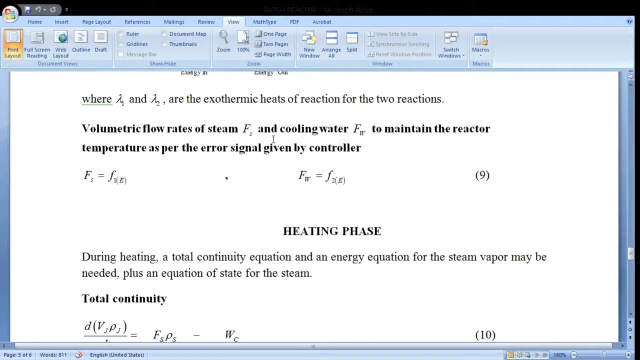 Here, energy in by the reactor here, And this is energy out from metal ball to the jacket, Inside the jacket here. So lambda 1 and lambda 2 are the exothermic heat of reactions, of two reactions Now, volumetric flow rate of steam and cooling water is just to maintain the reactant temperature. 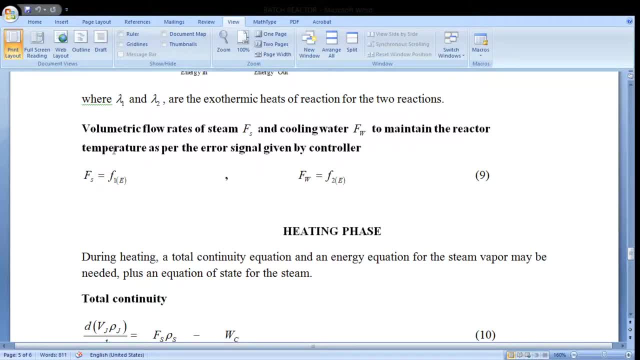 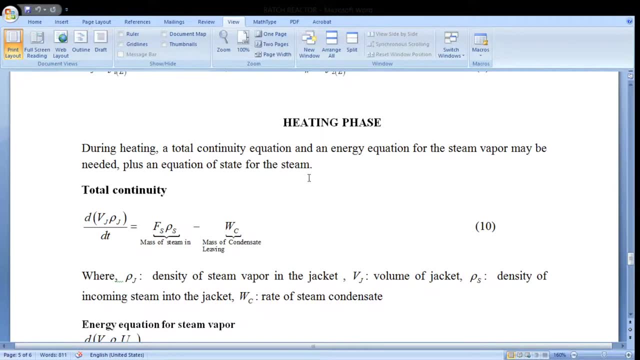 So they will have by the controller functions. So they would be given some control equations for stream and cooling water During the heating phase. in the beginning steam vapor is need to maintain the reaction temperature, So in the starting. So you are feeding a 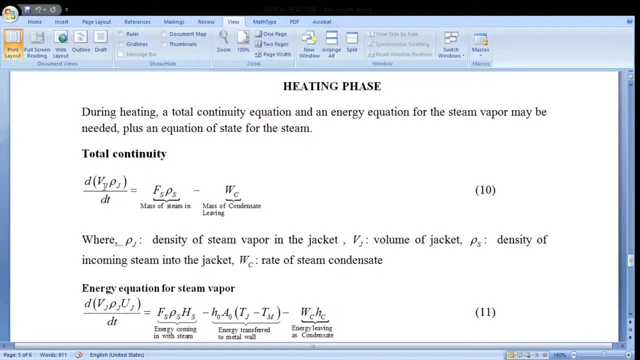 A volume of the steam into density And this is the feed rate, Mass rate of the steam in Fs into density And the mass of condensation: Condensate steam Leaving the jacket actually. So this is volume of jacket which completely fills density. 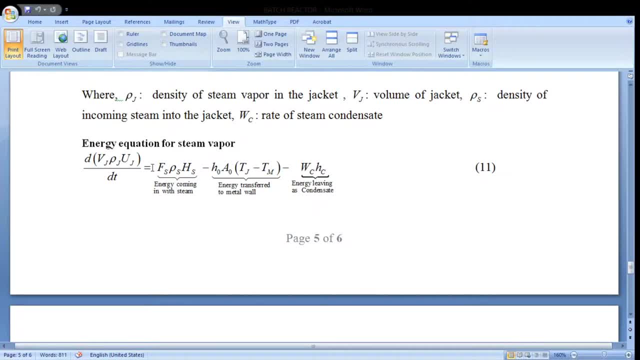 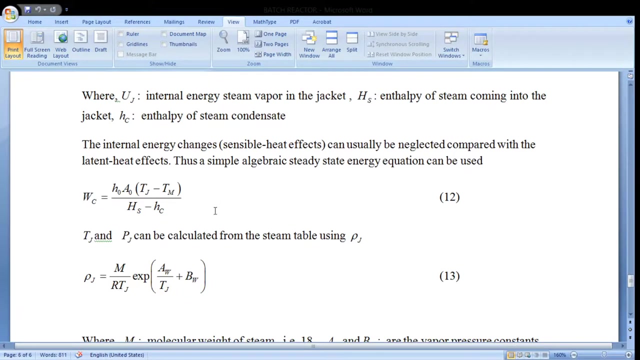 Then energy equation for the steam vapor. So this in terms of internal energies. So you are just balancing here: Enthalpy coming in with the steam And this is the energy is coming, Transfer to the jacket, to the metal ball, And this is energy going out with the condensate. actually. 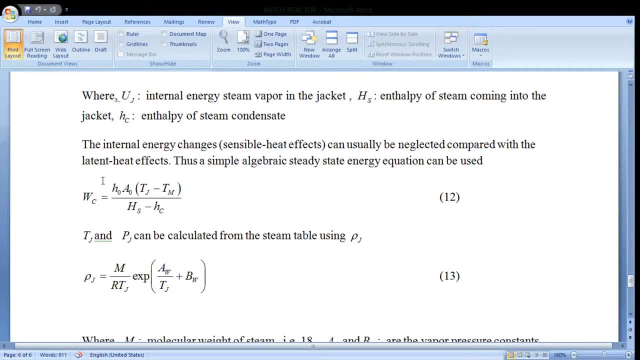 Now for the steam. You have one Another equations in terms of enthalpy of steam, Enthalpy of condensate And mass of the condensate, And this is some equation actually. So this is just to balance. Then density can be calculated from here. 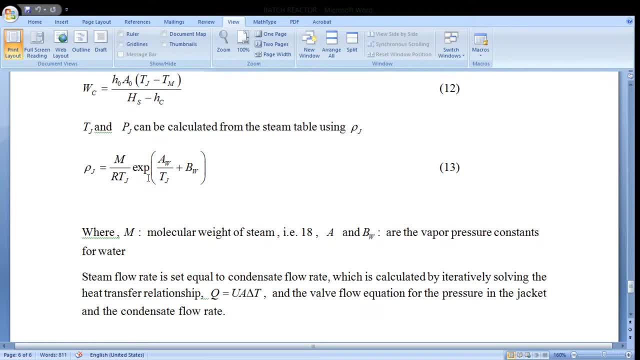 From this steam table. So this density of the steam That m upon r, t, j, Exponential a w upon t j, B w. A, w and A and b w Are the vapor pressure constant For the steam vapor. So this is the density of steam. 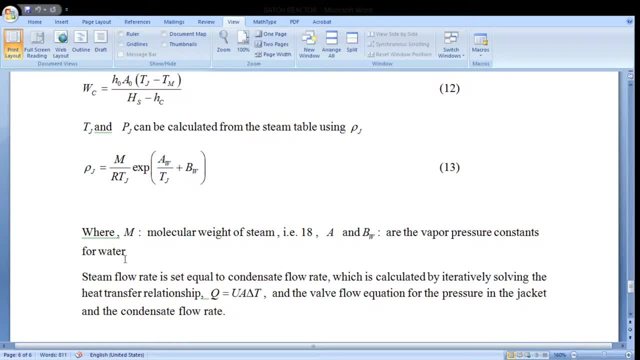 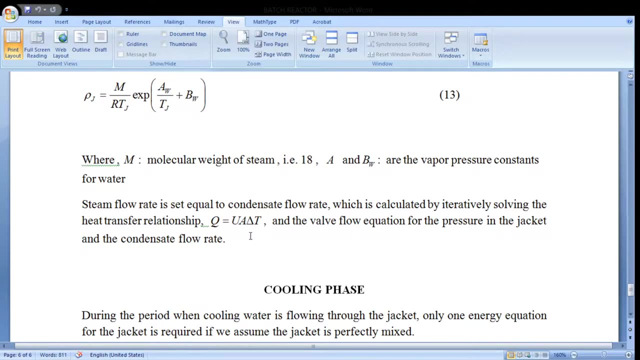 So this is the density of steam For the vapor pressure constant For water, M is molecular weight of the steam, Practically 18 actually. So this way, Then, finally, we are calculating The q equal to a delta t Condensate flow rate. 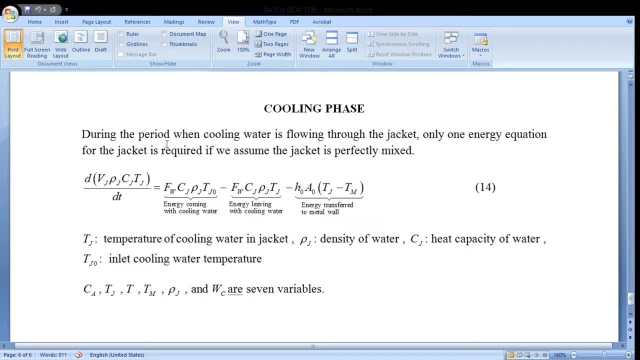 And in cooling phase Of jacket here. If you are saying There is a jacket here, So this is m, c, p, d t Of the jacket here. V? j into Rho j. The mass of steam in the jacket, The heat capacity. 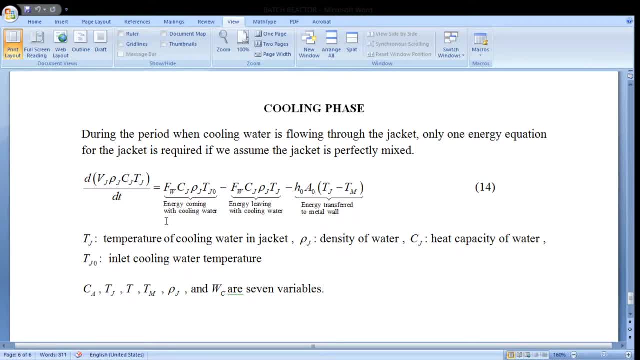 And this t j Inside jacket. So energy coming in with the cooling water, Leaving with the cooling water And energy transfer to the jacket, To the metal wall actually. So this is the For cooling phase actually. So you have initially 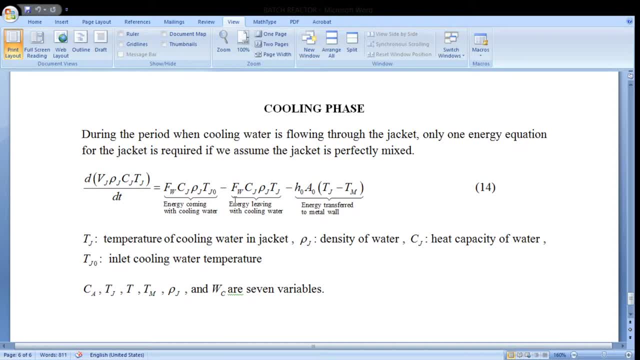 The heating phase, Then followed by The reaction Once the reaction has been Started, And then you have reaction, kinetics And total. you have 14 equations, And all of them Can be solved simultaneously. Some of them Would be clubbed here.